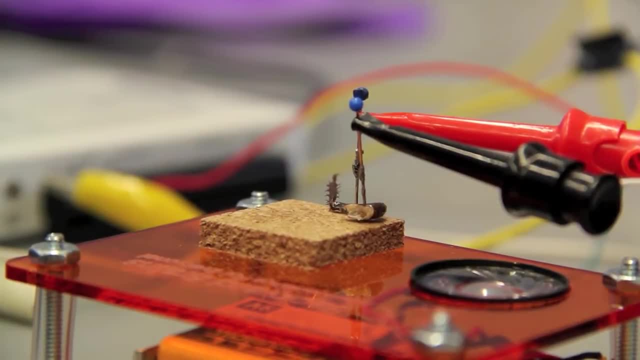 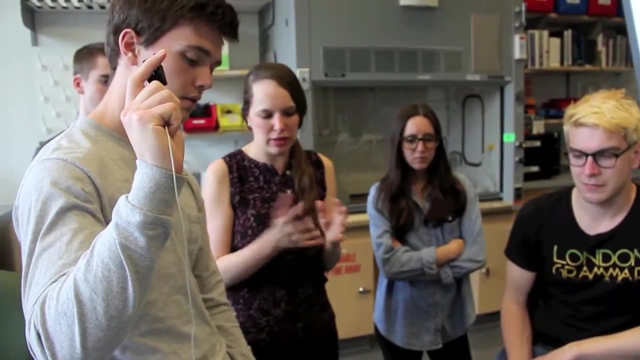 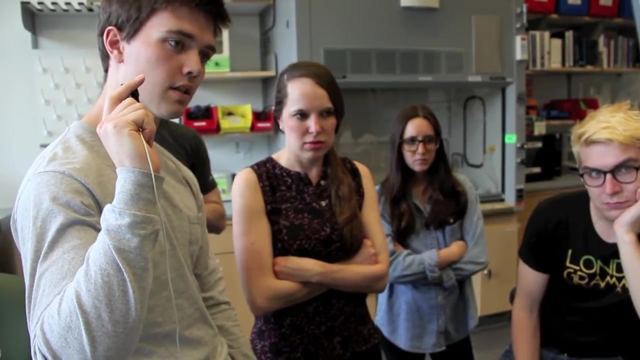 Yay, you got it right. Excellent, Okay, thanks, guys, looks great. I am Shauna Dorsey. I am the professor for this course, which is our junior level lab, And here where it gets really exciting is they're getting the opportunity to use biological systems. So I'm 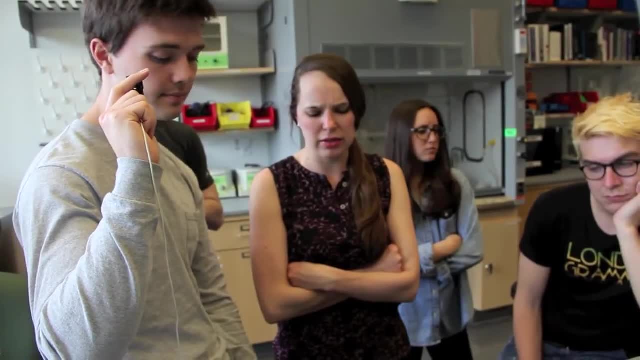 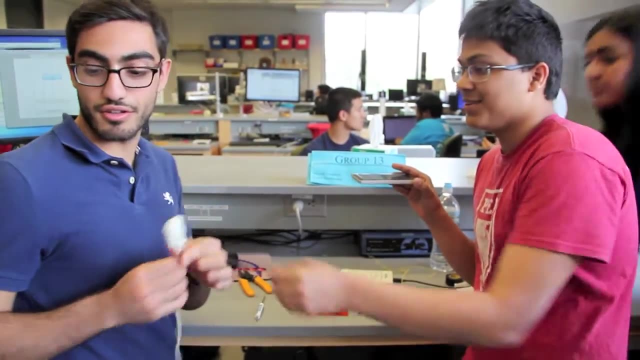 sure you've seen they're taking physiological inputs from their body, whether that's you've had different voice commands. we have different claps that students are doing. we have different brain waves. they're recording and then sending that into a physiological creature- In this case it's a cockroach leg- and seeing the output. 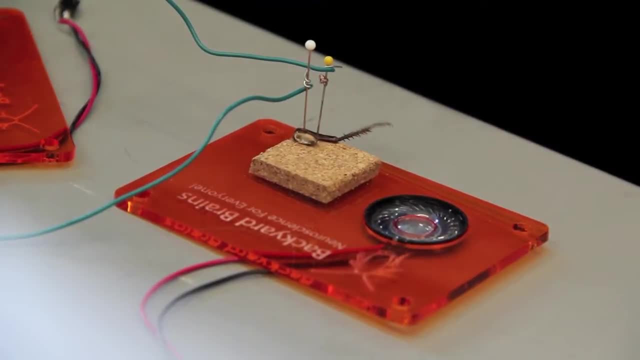 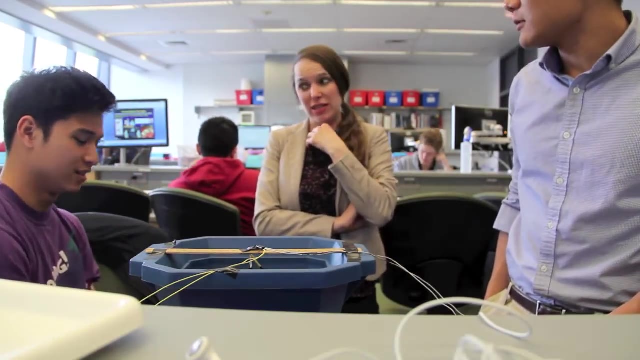 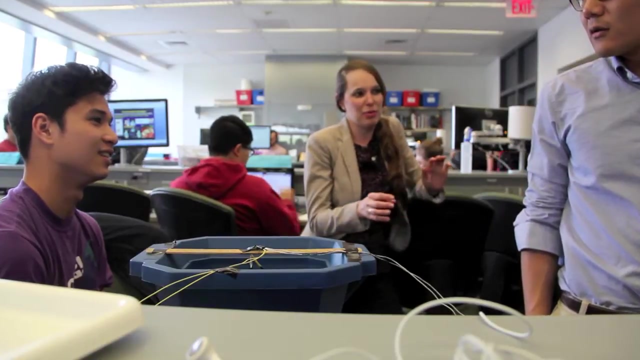 One of the biggest applications is in neuroprosthetics, So you can have a patient think about wanting to move his or her prosthetic arm and actually causing that movement. So that's really people having to retrain their own brains here to think of how to use prosthetics. 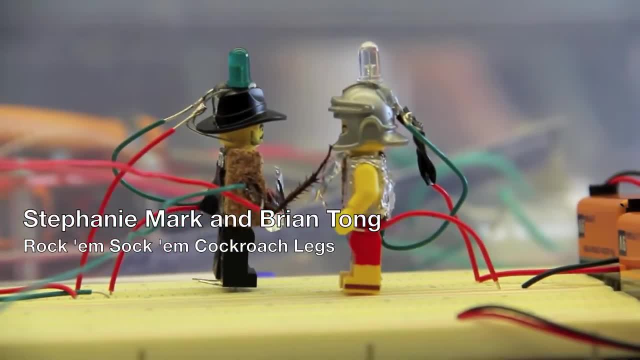 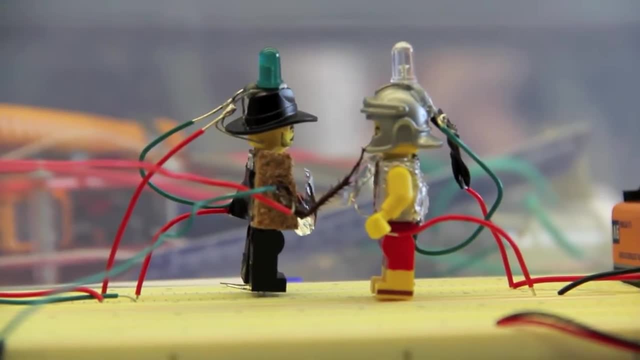 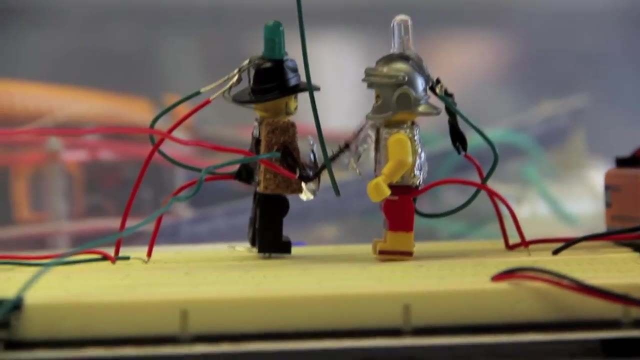 Once they're hooked up. I think we're gonna stick to one leg for now and just test to see whether our accelerometers will result in the desired cockroach leg movement and then, if it does work, then this little guy will light up to show that he's been hit. 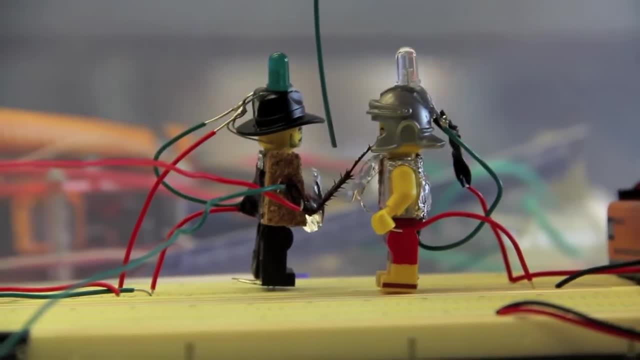 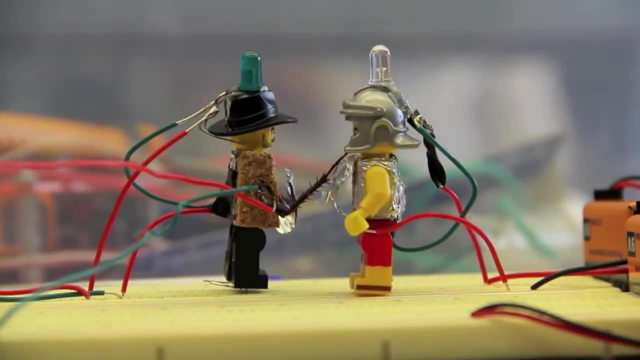 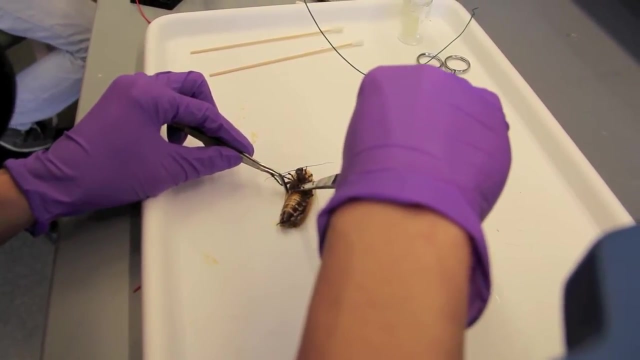 I think our enthusiasm kind of made us overlook some of the challenges involved in in completing the project, but I think we're getting there. I think we're getting there. Cockroaches have all of the features that you would want in engineering a system, so it's a limb. 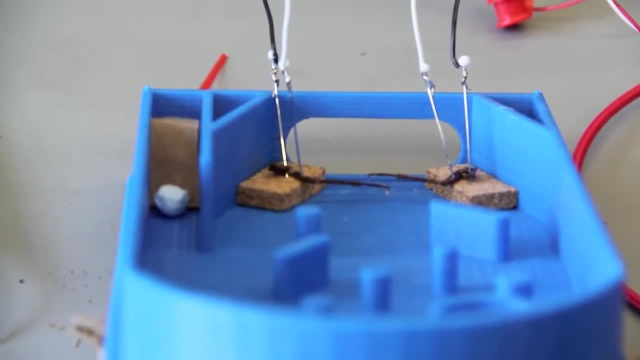 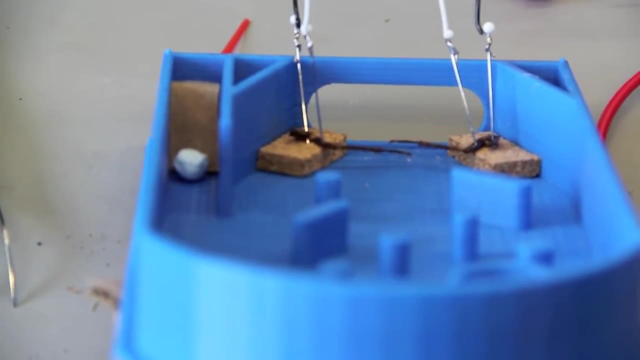 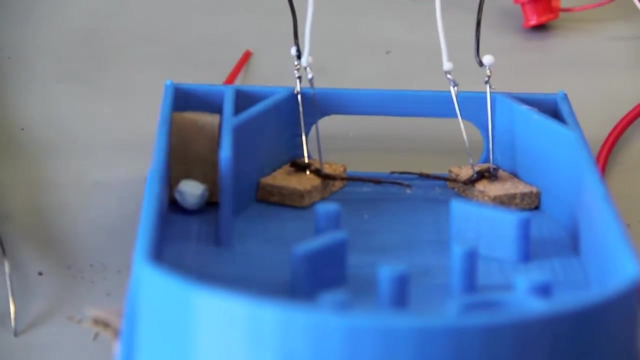 that can create complex movements based on the signal that you send to the limb. you can create one type of movement with a particular signal and then vary that signal to create an entirely different type of movement. so the flexibility of the movement and it's also simple enough so that it can be done on a project. 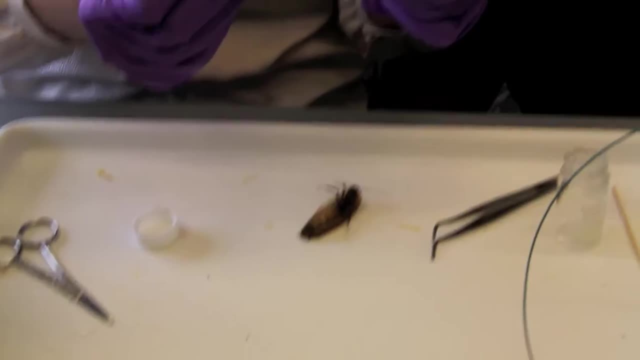 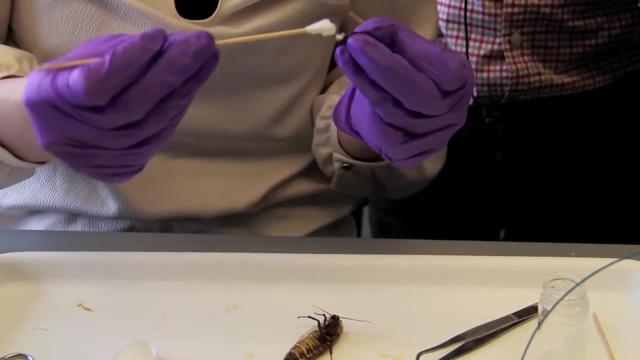 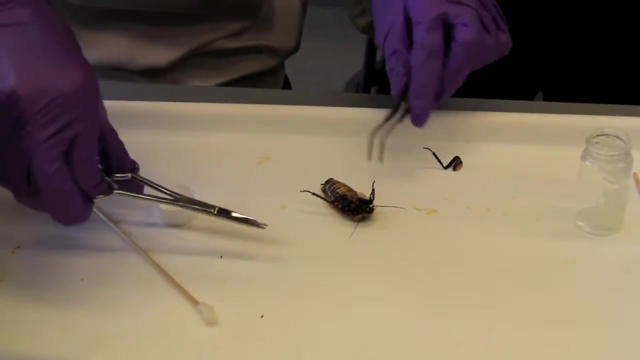 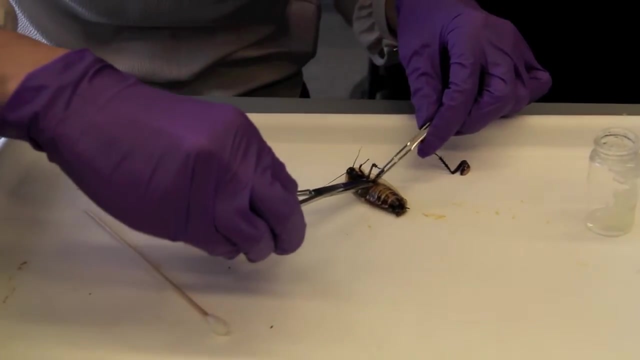 basis. over the course of a half a semester, I would say I've taken off about maybe eight legs so, and sometimes the legs switch just as a reaction, which is kind of unsettling. but I'm definitely less squeamish after this lab. we try to work as quickly as we can so the cockroach doesn't come out of its. 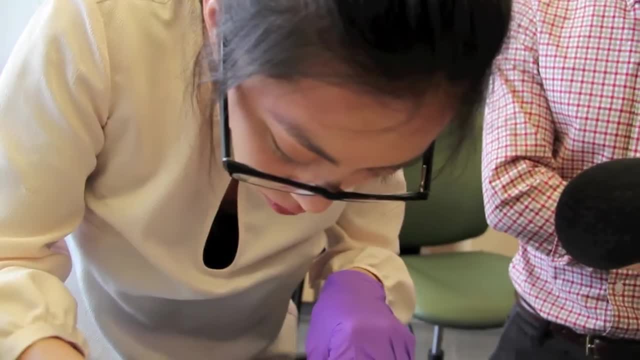 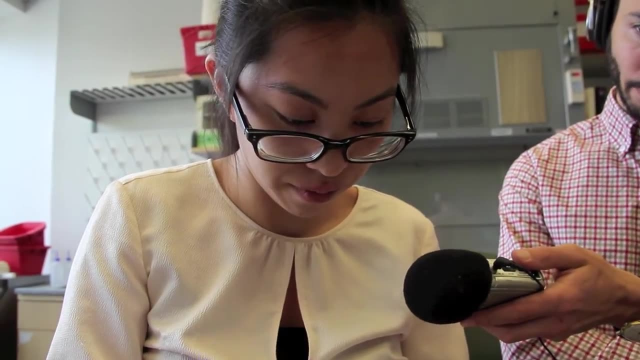 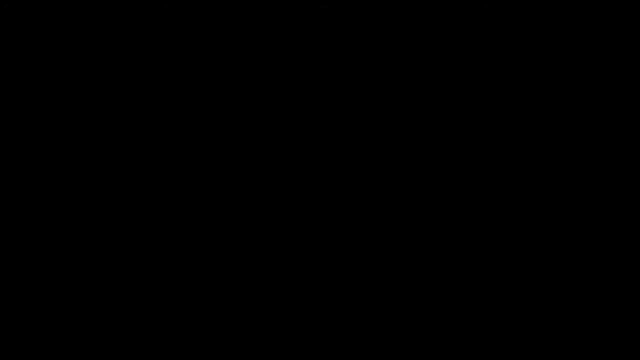 anesthetized state, then we're just gonna put him in a plastic bag and put him in the freezer to euthanize him fully. do they have tears? do you see cockroach tears over? I feel them in my heart but I don't see them.